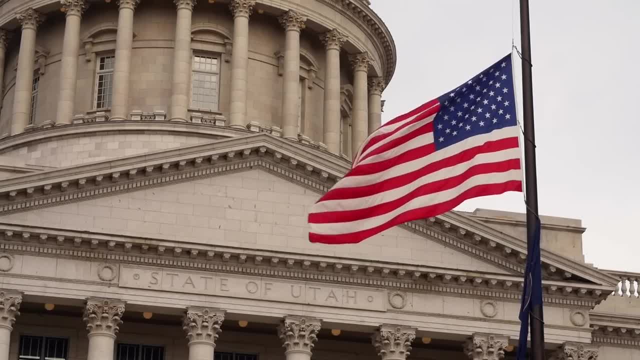 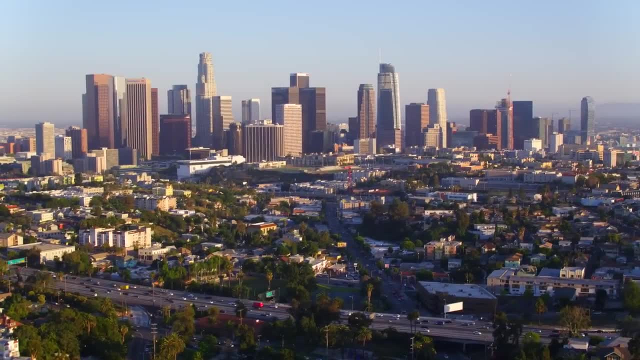 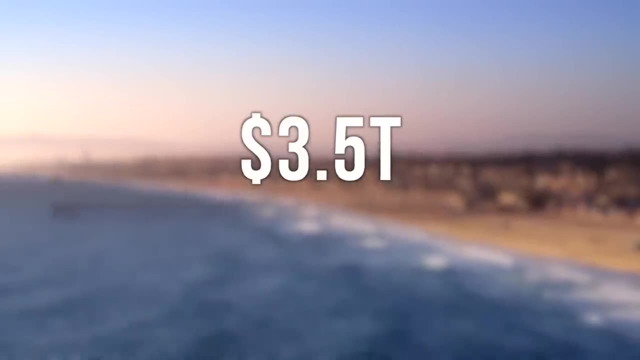 tropical paradise island. So how do the US's states compare to other countries of the world? Well, let's first start off with the big one. the US's richest state in terms of GDP: California. At a mind-blowing 3.5 trillion US dollars, California is by far the richest state. 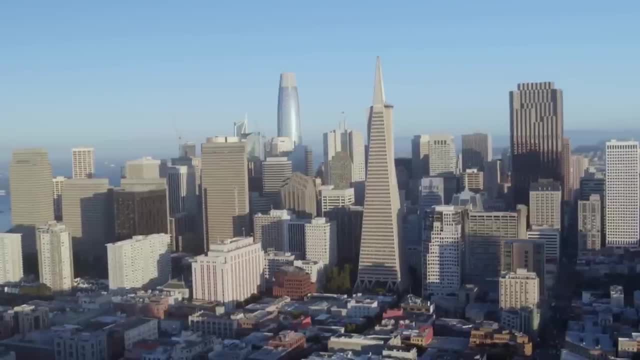 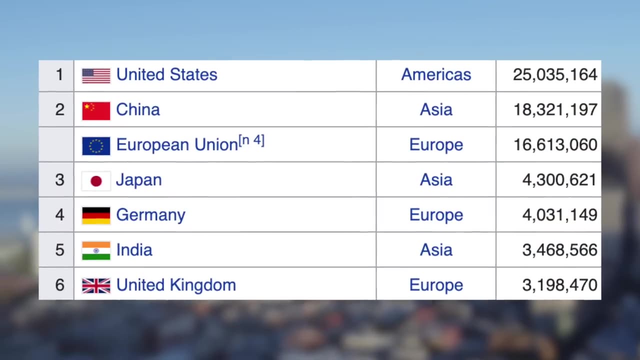 in the United States by economy size. The US is the richest state in the United States by economy size. If California was to remove itself from the United States and become its own individual nation, it would rank as the 5th largest economy on the planet, placing them just above India. 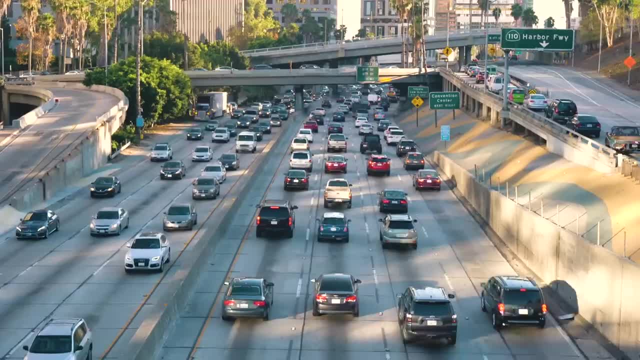 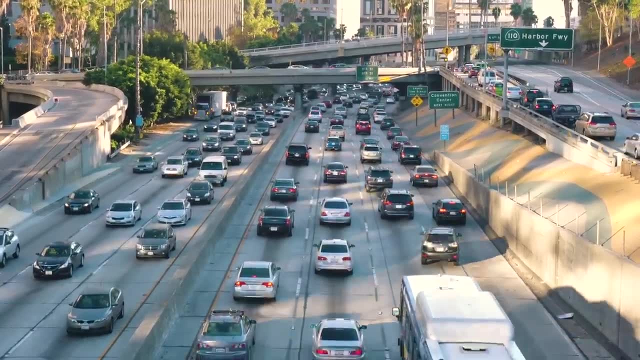 again a country with over 1.4 billion people. California's total population is just shy of 40 million, around the same as Canada or Greater Tokyo. California's wealth comes from a variety of sectors, but most importantly from Silicon Valley, the home of the 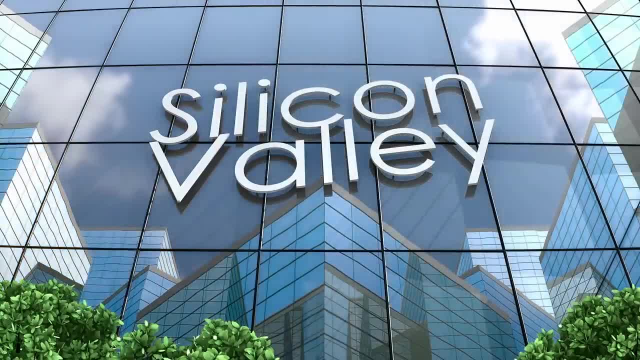 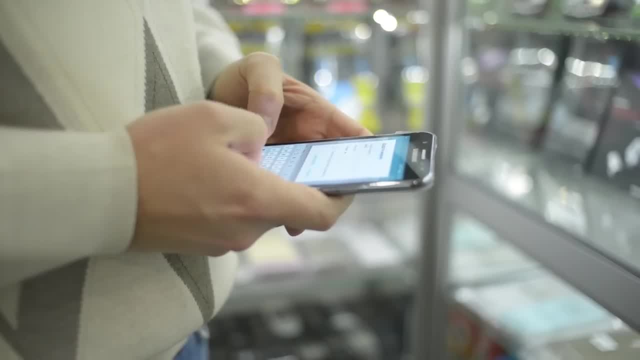 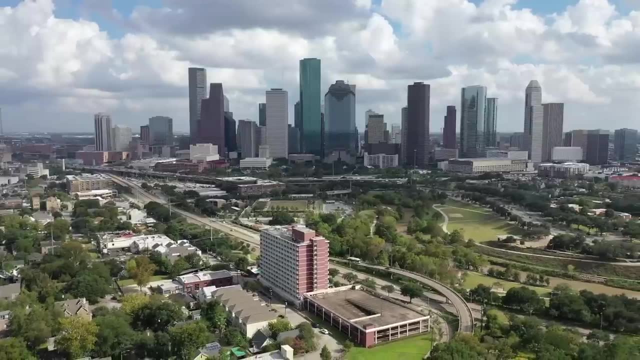 tech corporations that essentially run the fabric of humanity. Decisions that are made from the companies that reside in the state quite literally change the shape of our planet and influence billions of people. At 2.3 trillion US dollars, Texas ranks second as the state with the highest. 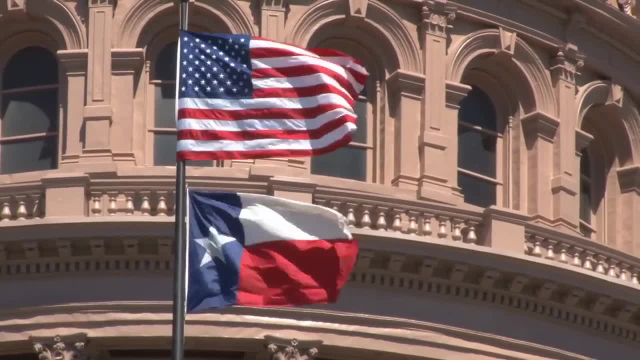 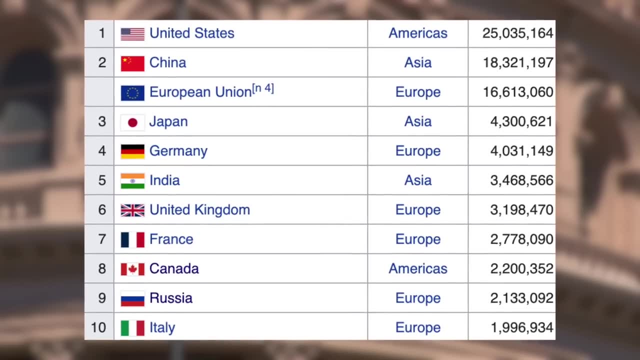 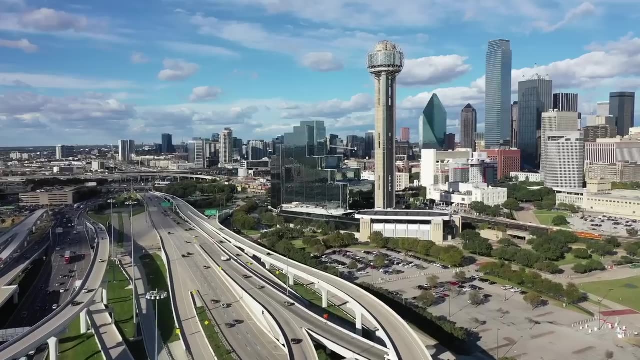 GDP in the United States. Again, if Texas were its own country, this would rank them as the 8th largest economy in the world, placing them above the likes of Canada, Russia and Italy. Texas' population is only 30 million, meaning that the state punches well above its weight. 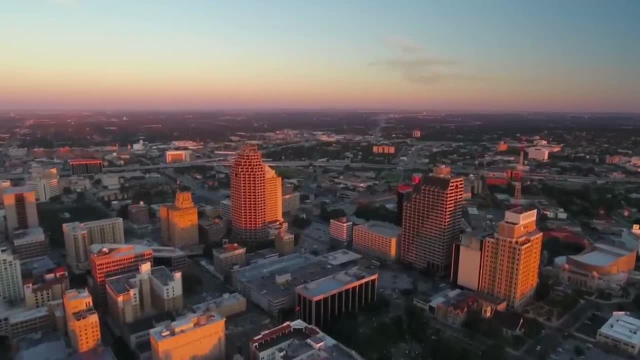 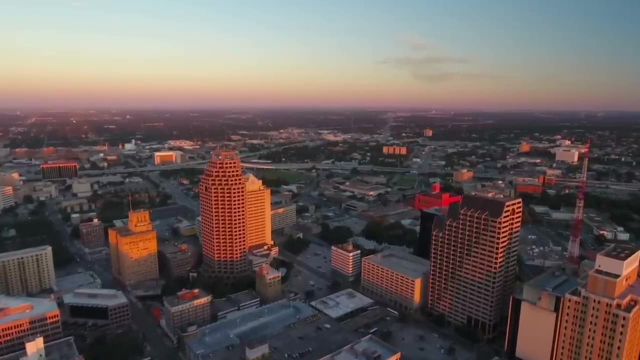 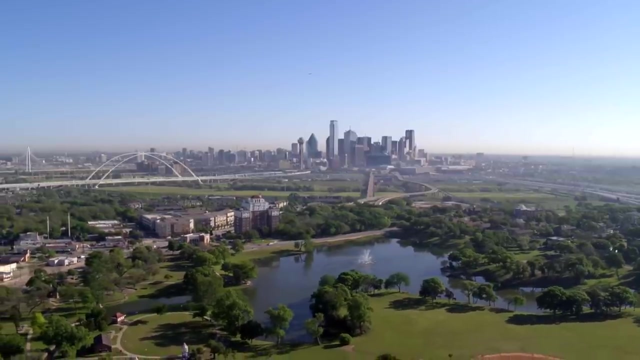 in terms of wealth. This 30 million population would rank Texas as the 49th most populated country in the world, yet it would easily rank in the top 10 for its GDP. At nearly 700,000 kilometers squared, Texas is the largest state in the contiguous US. It is completely dwarfed. 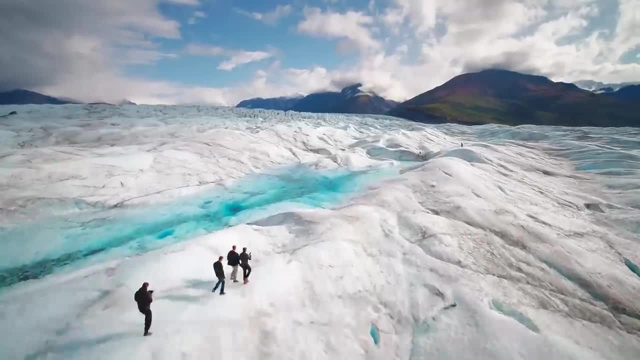 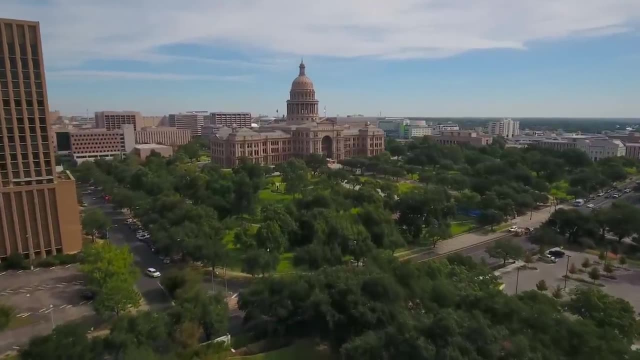 by the US's largest state, Alaska, which is around 1.7 million kilometers squared. Texas is so big that, if it were its own country, it would rank as the 39th largest in the world, largest than Myanmar, which is the second largest. 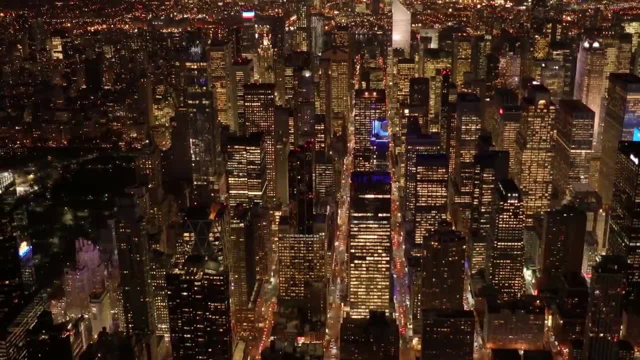 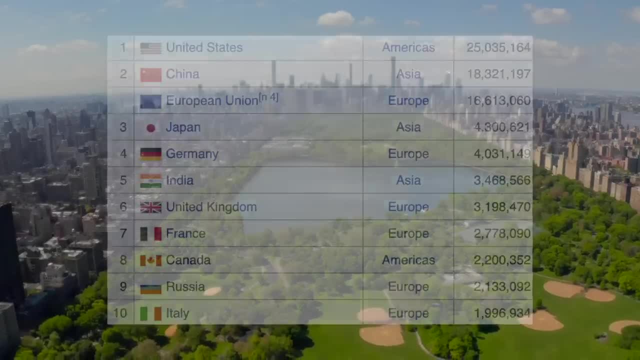 country in Southeast Asia. New York State comes in third place for the richest state by GDP, at just over 2 trillion US dollars. This would see them rank in the top 10 for the largest economies on the planet, placing them just above Italy. New York State is of. 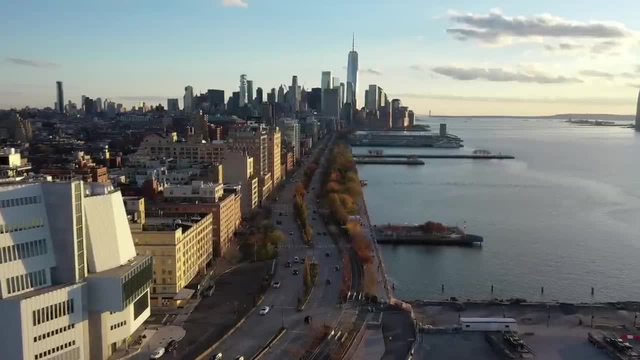 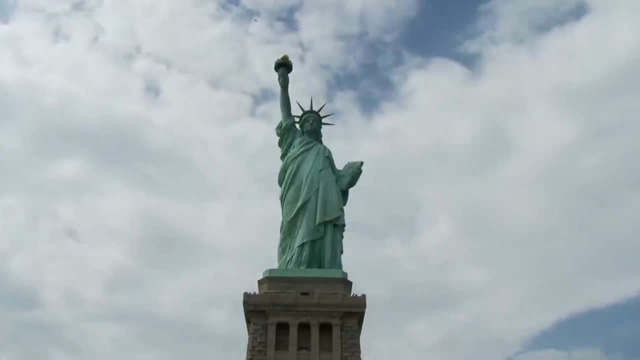 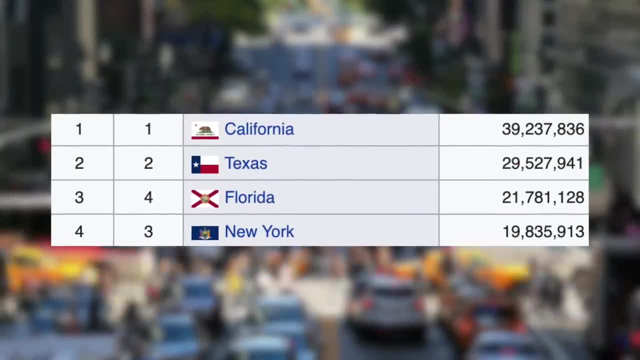 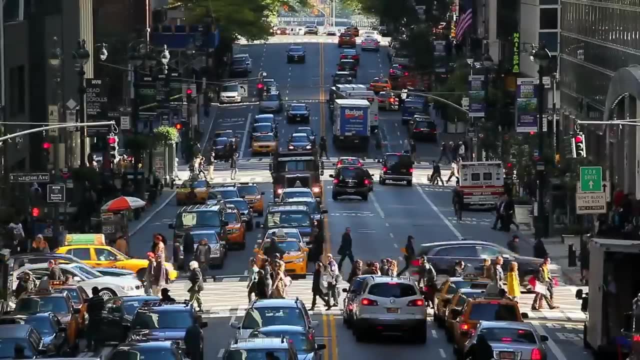 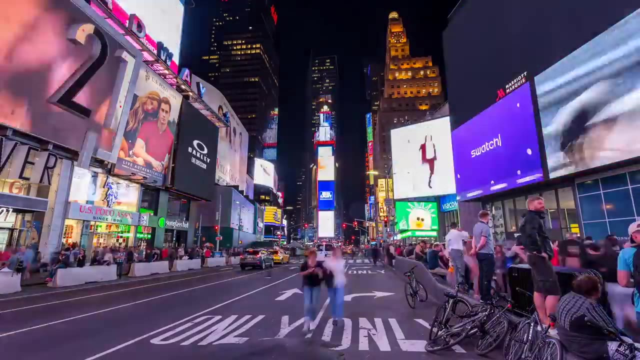 planet At 20 million. it is the 4th most populated state in the US and the second richest in terms of GDP per capita, at over 100,000 US dollars. This 20 million population would see New York State ranking as the 62nd most populous country on Earth, placing them just. 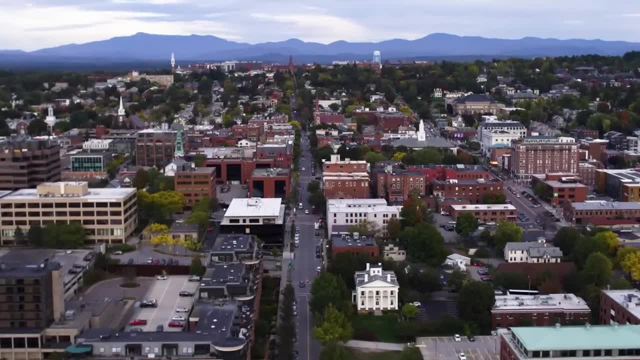 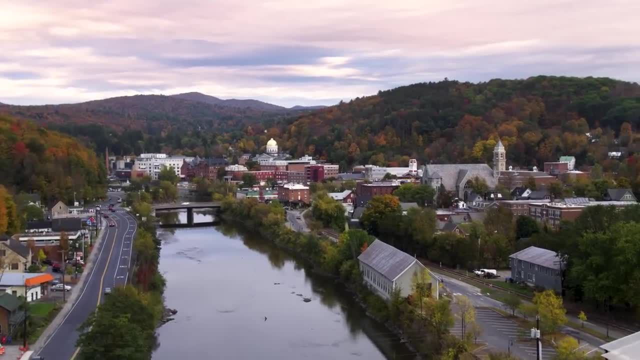 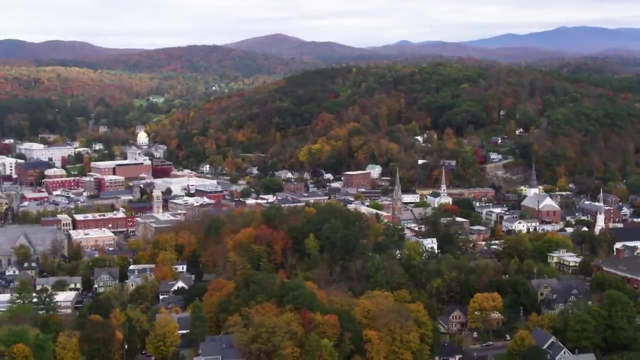 above Chile. Vermont ranks as the state with the smallest economy in the US, at just 40 billion US dollars, partly due to being the second least populated, with a population of around 650,000.. So where would an economy size of 40 billion rank Vermont in the world? Well, it's not as bad as you. might think It would see them just ranking outside of the top 100 richest countries in the world by GDP, in 101st place, eclipsing the economies of Latvia and Estonia, two European countries with much larger populations. Vermont is also pretty darn small ranking as the 45th largest state in. 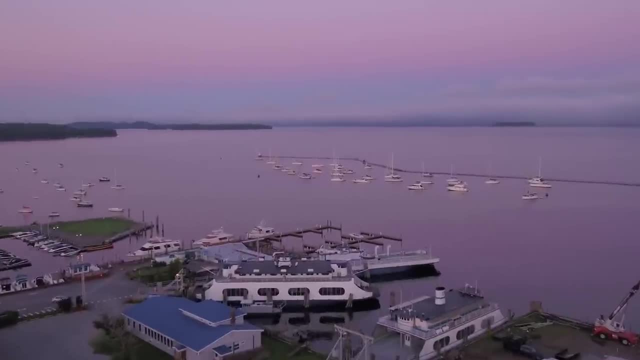 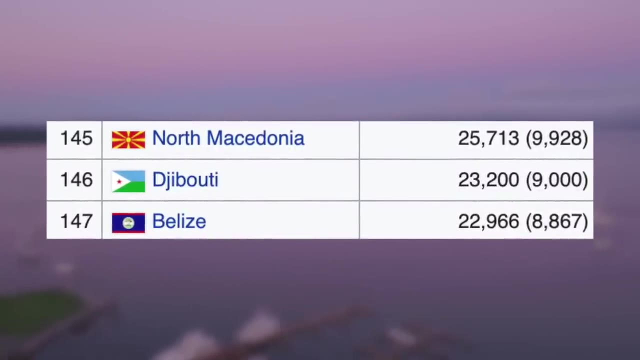 the US at just under 25,000 kilometers squared. This would rank Vermont as the 146th largest country in the world if it was its own individual nation, placing them above the likes of Djibouti, El Salvador and the Philippines. 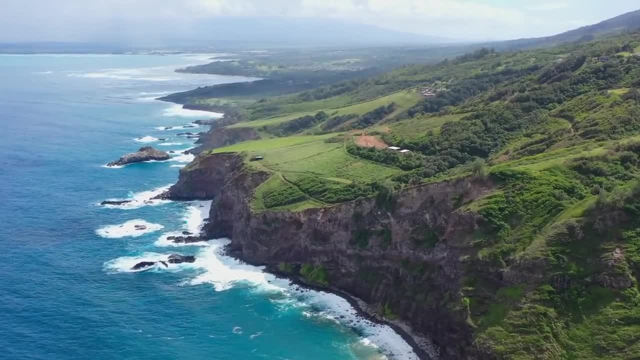 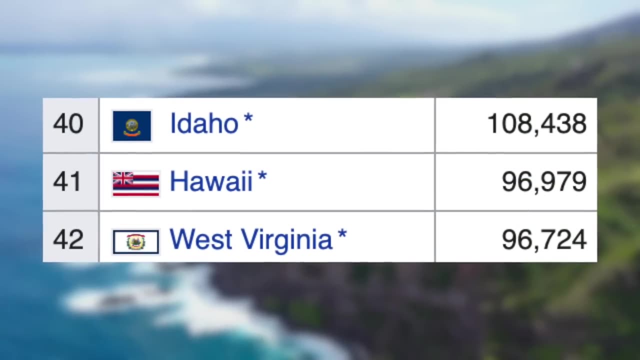 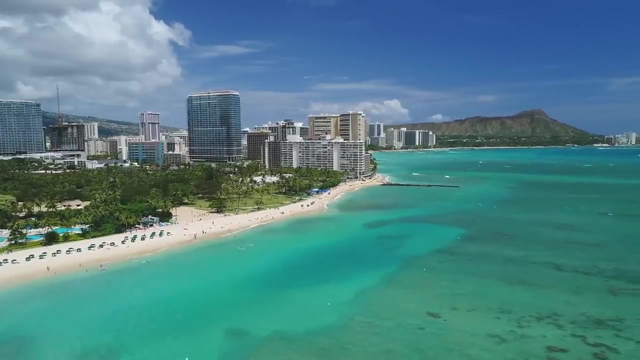 Hawaii, which is quite possibly the most dreamy US state to visit or live in, ranks as the 41st richest in terms of GDP, at just under 100 billion US dollars. This tropical paradise would see themselves ranking as the 69th largest economy in the world, Alongside Alaska. it is the only US state. 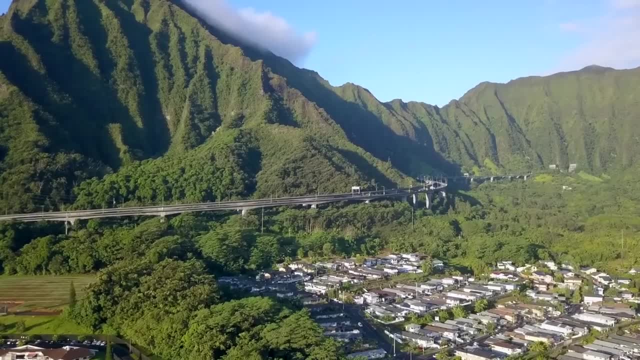 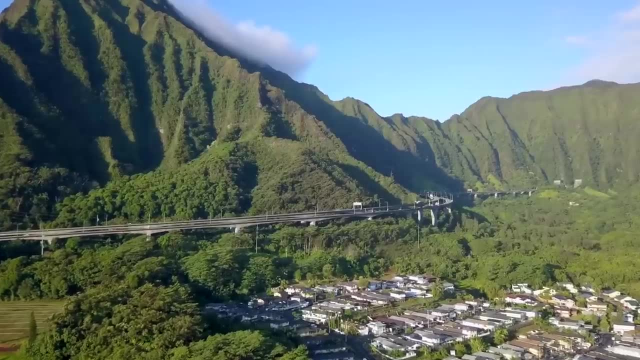 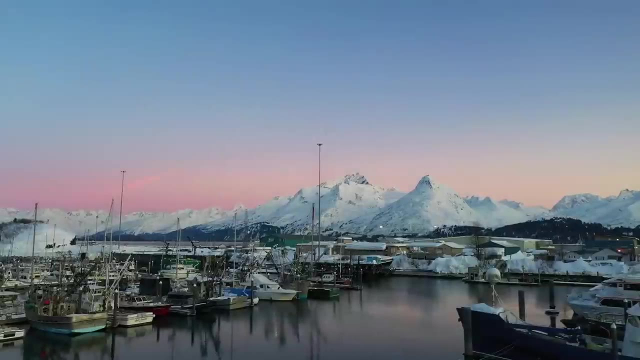 not connected physically to the mainland. Just 1.4 million lucky people call this state home. This would rank them as the 151st most populated country in the world, around the same amount of people who live in San Diego, California. As mentioned earlier, Alaska is the US's largest state, at an incredible 1.7 million.